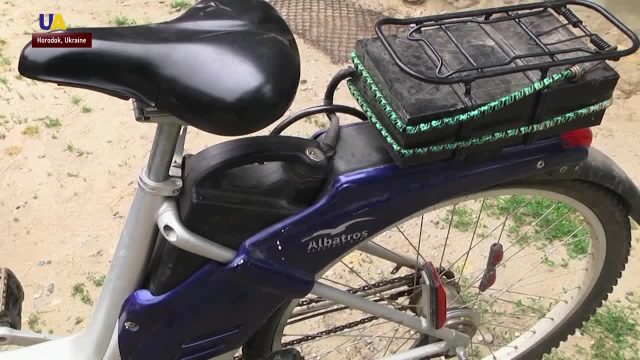 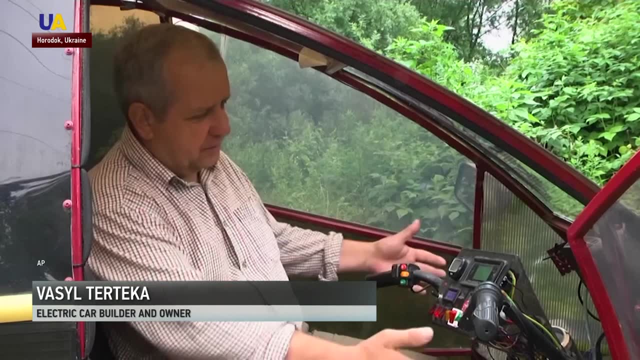 a small, economical car would be better suited to the job than an electric bike. I bought a used electric bike and remade it, fixed the engine and changed the accumulator, And I did it because I wanted to use it to go to my apiary. 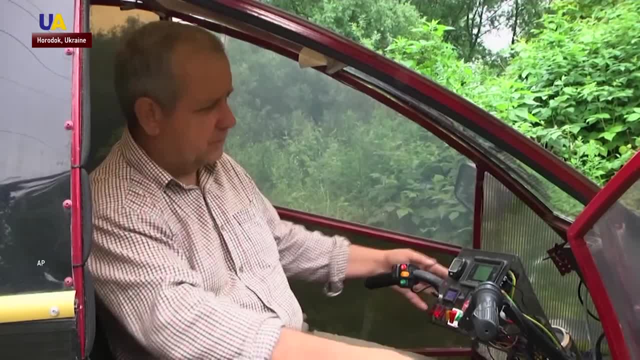 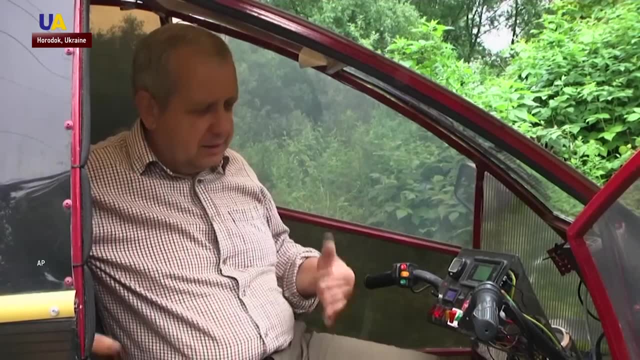 which is 25 kilometers from here. But it was a bit hard to drive such distances on a bike. I'm not getting any younger, So I decided to construct a little electric car. At least no wind is blowing into my face and no rain is pouring on my head- Much better than the bike. 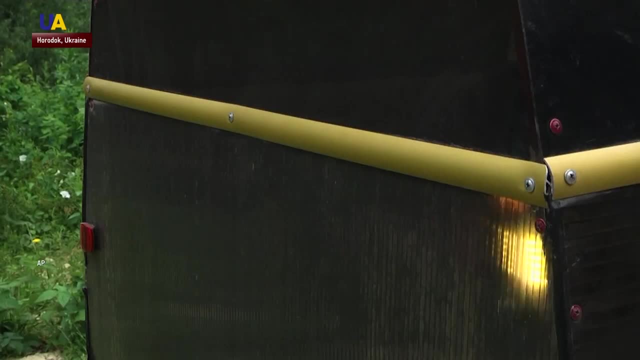 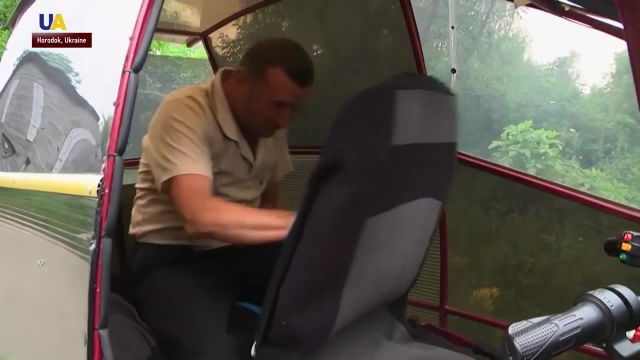 Terteka learned the basics of electronics 40 years ago on a radio mechanics course. He also taught himself some extra skills on the internet in order to build this car. The vehicle cost him 1500 US dollars to make. He says it now costs him just 10 euro cents to drive. 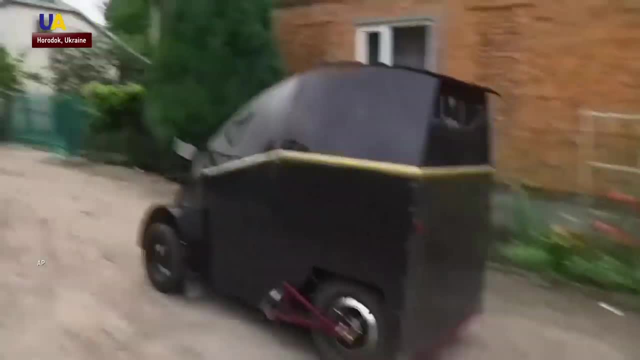 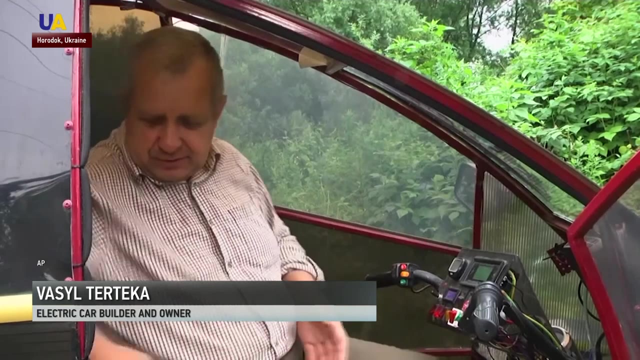 100 kilometers in his little car, Something that would cost at least 6.7 euros in a regular one. I had no drawings or plans. I simply started making the front suspension part and then, slowly, little by little, I made a carcass. 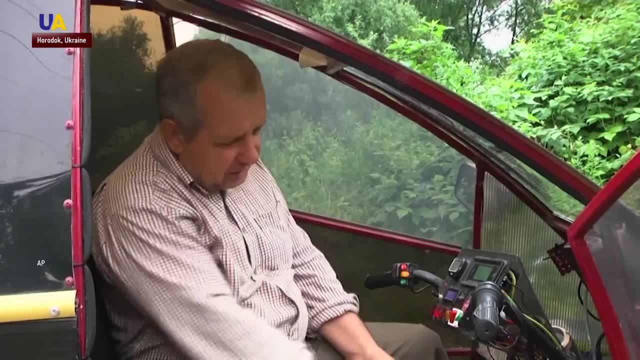 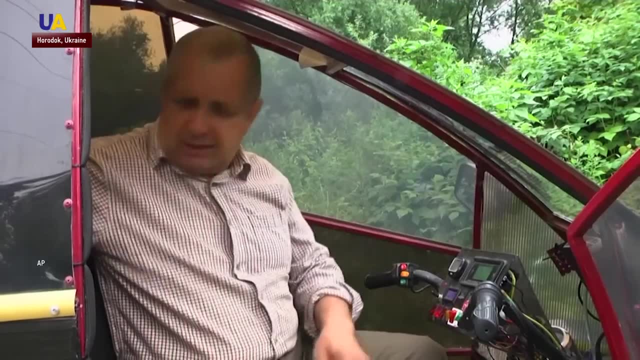 I left enough space here in front to fit in the accumulators, to make sure, oh, the weight doesn't fall on the back of the car, because there would be passengers too. I then tested what I had put together, and only afterwards I started covering it. 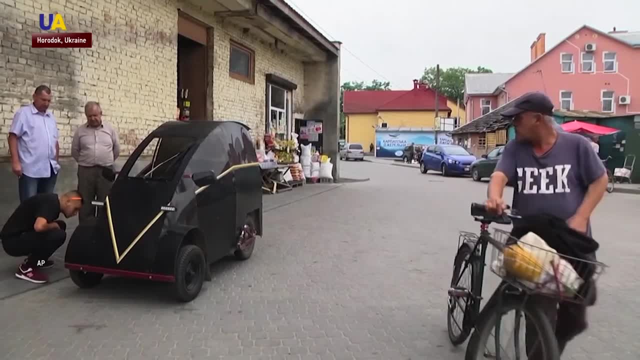 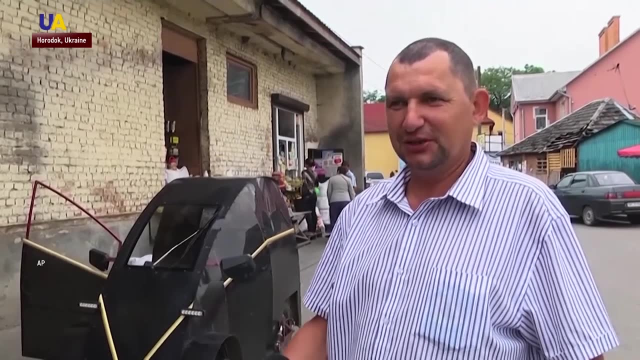 in polycarbonate plates. Although at the start many people didn't think you could pull it off, now they're lining up for test drives. It's neatly done and ecologically clean. No emissions at all. It is a very good car. 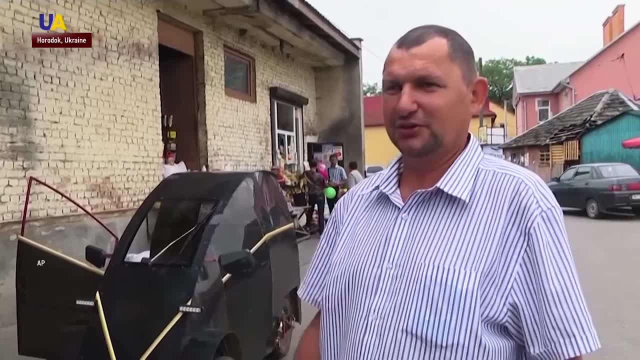 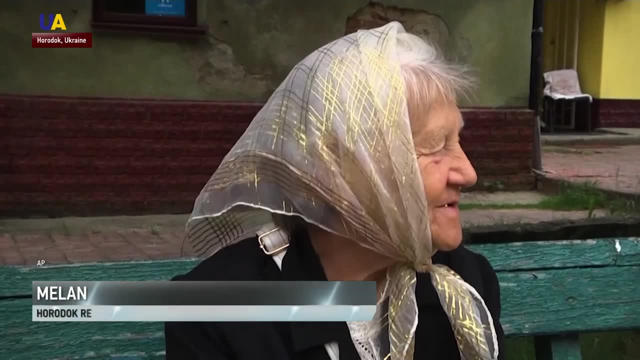 I wish I could buy a car like this one, but I don't have enough money. I've been looking at it and thinking whether someone could give me one too. Very nice and comfortable. It is small and can get around Here and there easily. 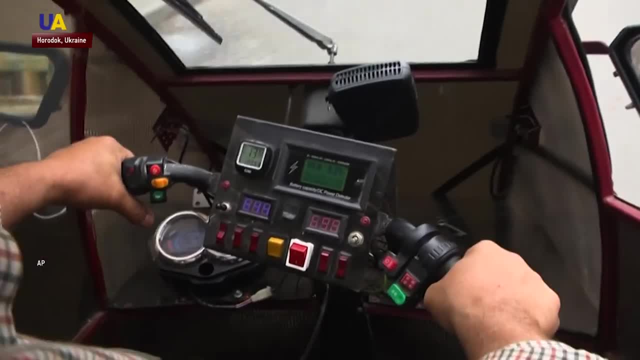 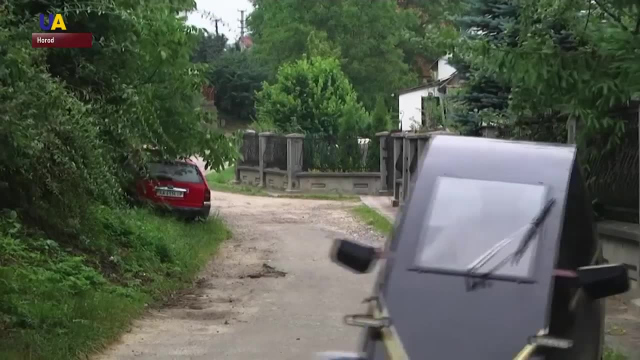 The car is very compact but can fit another passenger. It reaches a speed of up to 58 kilometers an hour and can go for 100 kilometers on one full charge. The inventor has been asked to sell the car multiple times, but is resolute that this one's all for him.